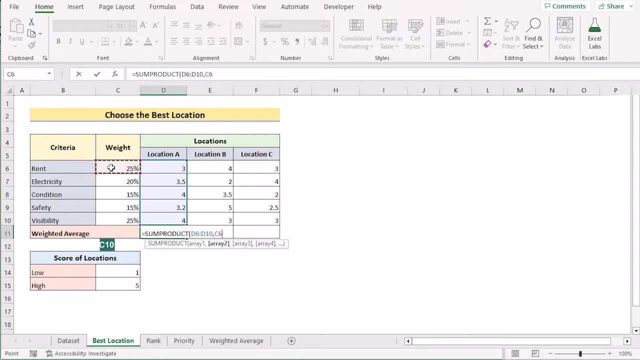 by which we want to multiply the cell. We'll select c6 to c10 and to make it permanent we'll use f4 in the keyboard. After that we'll divide the whole sum product by using the sum function. The sum function literally adds all the selected cells, So I will go for the c6 to c10 cell. 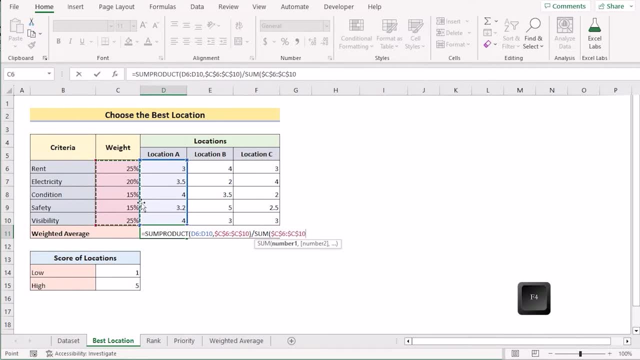 and now we'll make it permanent by using f4 in the keyboard. If we click the enter button, then we'll get our perfect weighted average for the d11 cell. You can drag the formula from left to right to get results for every cell. So that's how we can easily get the weighted average by using the. 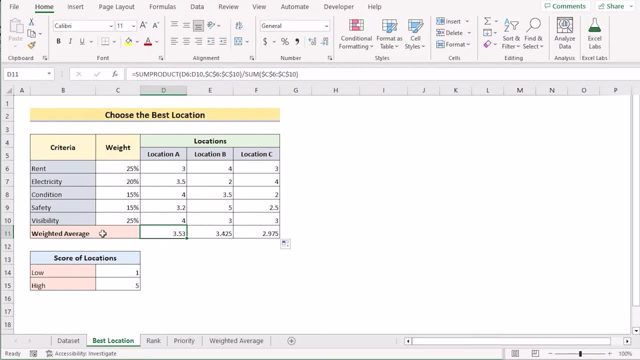 sum product and sum functions. Now, the location of the sum product function is the same as the location a. Location a have weighted average of 3.53.. Location b have 3.42 and location c have 2.97.. Among these three locations, the highest weighted average is for the location a, So it is the best. 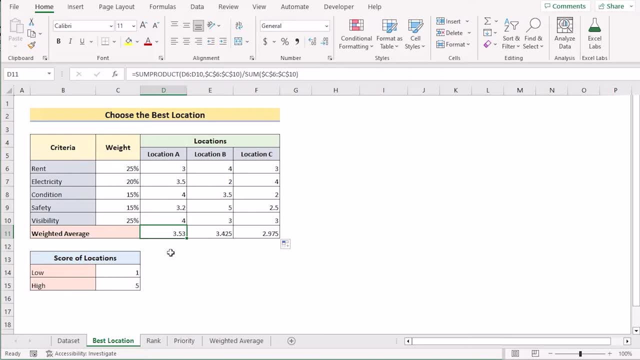 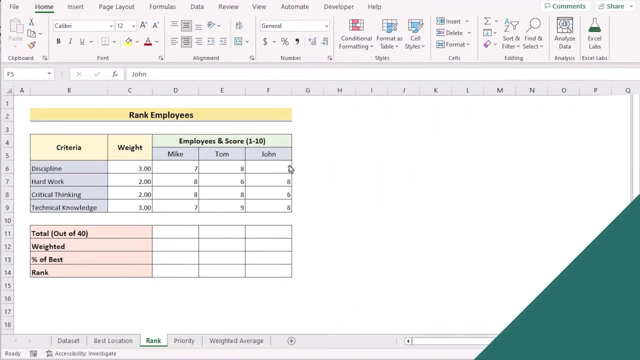 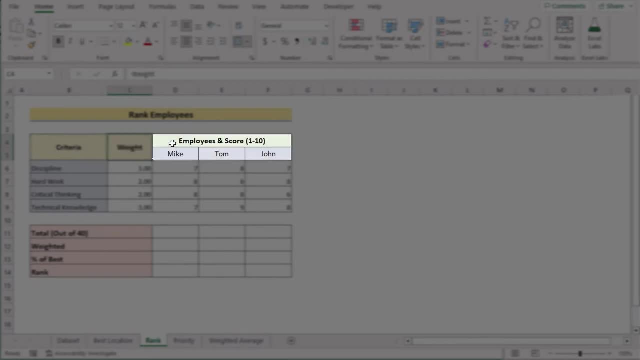 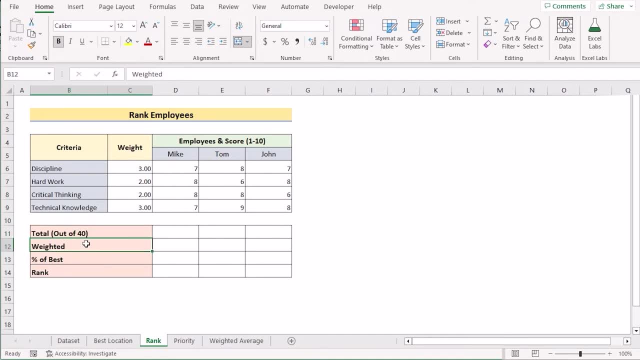 and f. We have total weighted percent of best and rank. in the b11,, 12,, 13, and 14 cell We'll be using sum, sum, product max and rank functions to rank the employees. So at first we'll be going. 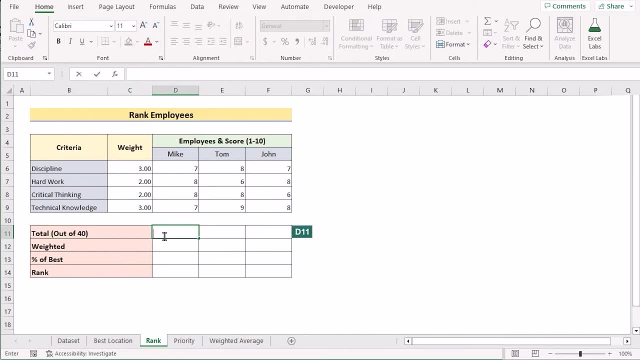 at the d11 cell and we'll insert the sum function to sum all the values here. We'll select the d6 to d9 to get the result for the first employee, Mike. We'll drag down the formula from left to right to get the same total number for Tom and John in the e11 and f11 cell. Next we'll move on to the. 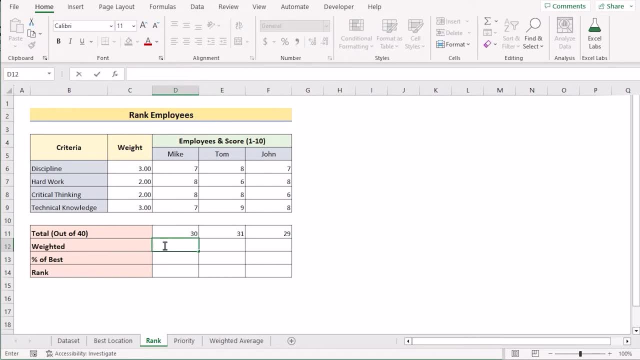 weighted section. Here we'll be using the sum function to rank the employees. So at first we'll be using sum product. So we'll write down the sum product function, which basically returns the sum of the products of corresponding ranges or areas. We'll select our first area here, which is in this: 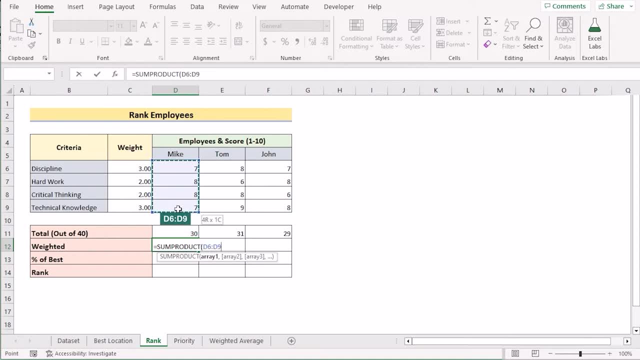 case, from d6 to d9.. In our next section we'll go for the weight, which is, in this case, c6 to c9.. And to make it permanent, we'll be using f4 in the keyboard. If we click the enter button, we'll get. our perfect weightage here. Next we'll be using the sum function to rank the employees. So at first we'll be using the sum function to rank the employees. So at first we'll be using the sum function to rank the employees. So at first we'll be using the sum function to rank the employees Now. 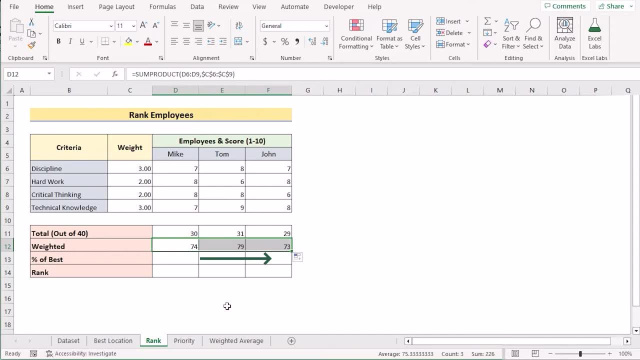 drag down the formula from left to right to get result for the three employees. Now we'll be moving for our d13 cell. We'll use first select the d12 weighted section and divided it with the max function. The max function returns the largest value. 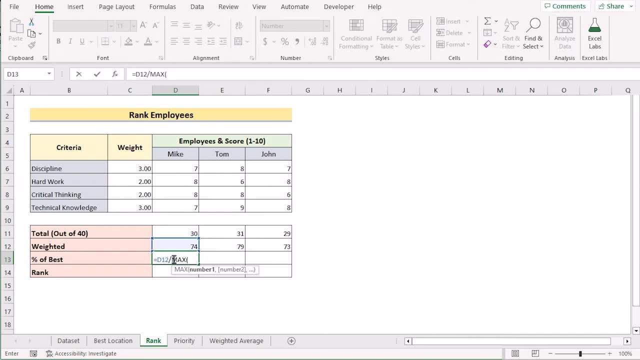 in a set of values. So we'll select the values here, which is in this case d12 to f12, and make it permanent by using f4 in the keyboard. Now we'll click the enter button to get the percentage of best here. Drag down the formula from left to right to get result. 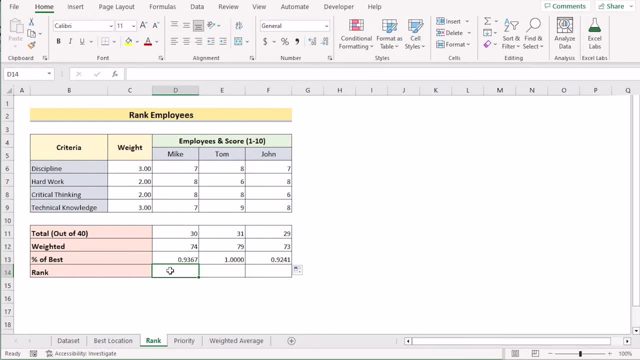 by using the weighted section. After that we're going to our last section. In this last section we'll be using the rank function, So we'll go to the d14 cell and insert the rank function. The rank function is the rank that we want to get the result for. 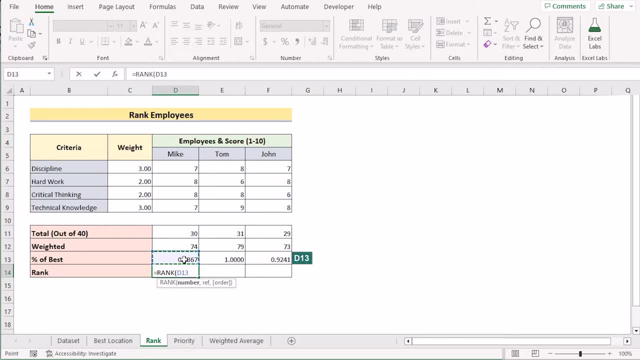 And now we'll be selecting the D13 and as our first number and going for the reference, which is, in this case, from D13 to F13, and make it permanent by using F4 in the keyboard. If you click the enter button, be getting the rank here. Drag down the formula from left to right to. 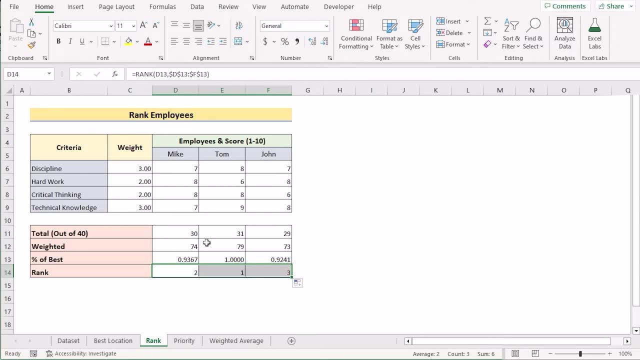 get the three ranks according to your wish, As the highest weighted have the Tom employee, so he has got the rank one. Who has got next value has got the second rank, and the lowest rank has got the John three rank. So that's how we can easily rank employees by using weighted scoring model in excel. 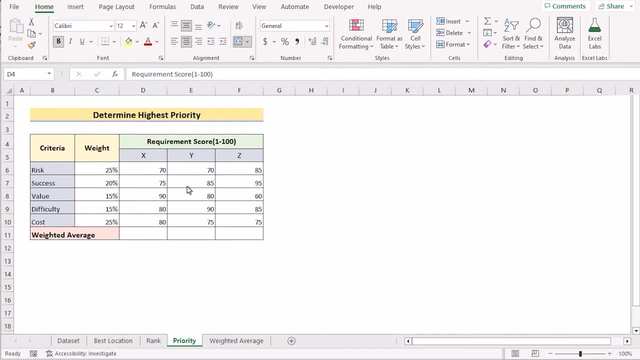 Now we want to determine the highest priority by using a weighted scoring model. To do that we have criteria, their weightage and requirement scores in between 1 to 100 of xyz in column B, C, D, E and F. Our target is to get the weighted average in the row 11.. At first we'll be 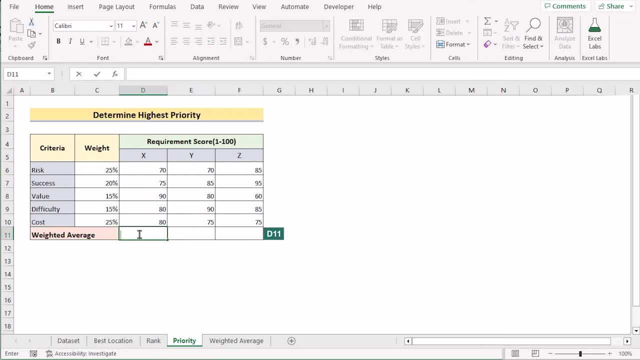 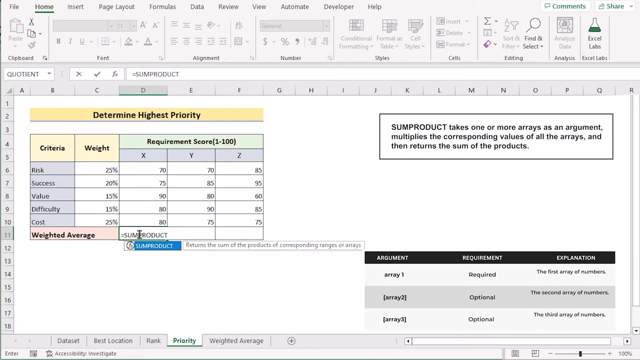 going to the D11 cell to insert the sum product and sum function. So at first we'll insert the sum product to D11.. To return the sum of the value of the corresponding ranges or areas. At first we'll be selecting our first array, which is in this case D6 to D10.. Now for the second array, we'll be selecting C6 to C10. 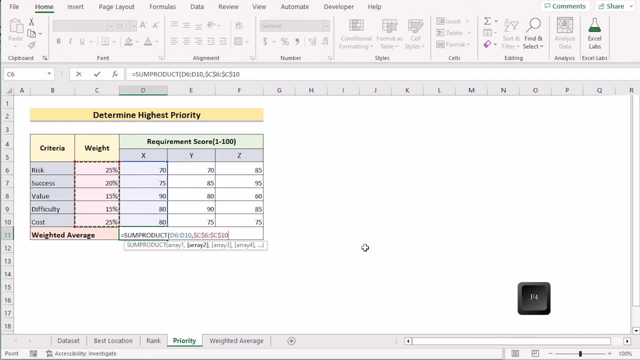 and make it permanent by using F4 in the keyboard. After that we'll divide it by the sum function. So write down the sum function to sum up all the numbers of the selected cells. We'll select C6 to C10 in this case and make it permanent by using F4 in the key board If we'll click the enter button. 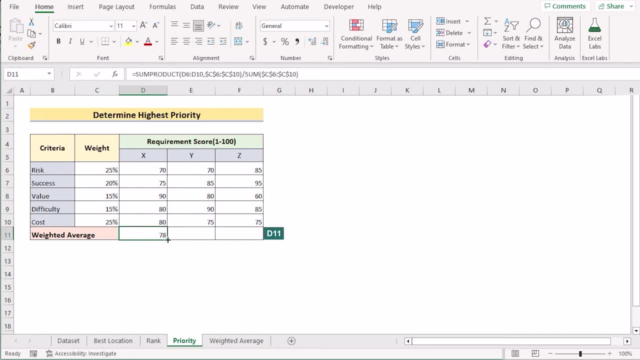 we'll get our perfect weightage in the D11 cell. Now drag down the formula from left to right to get result for the weighted average for every cell. Let's talk about result a bit Here. the weighted average of z has the highest value, But where the value of the x has the lowest weighted average. So 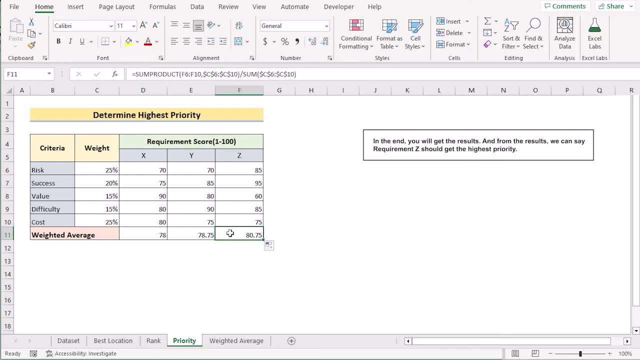 the highest weight in the dzie is 4.5.. Let's carry onto D processor. So D provents: every cell with a highest priority will be given on the Z and lowest priority will be given on X. So that's how you can easily determine the highest priority: by using a weighted.